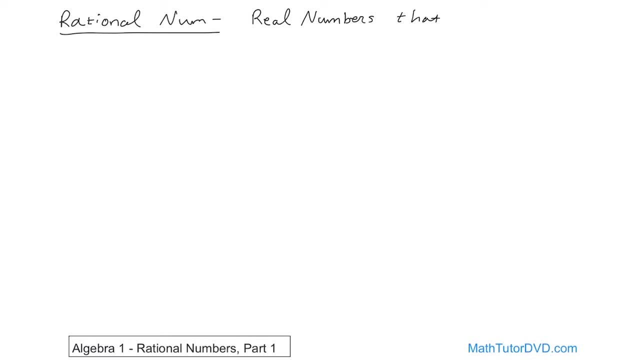 that means in just a second That can be written as a fraction. So when a number can be written as a fraction, we call it rational, because it's sort of planned by the rules. It's a well-behaved number, Well-behaved number. So let's examine this definition. First of all, we're saying that 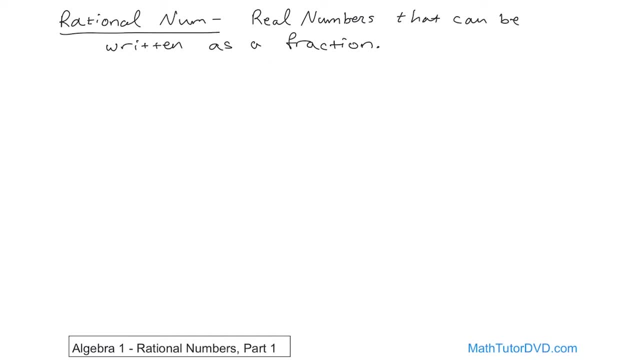 a rational number is a real number. Now, we haven't talked about imaginary numbers yet, but when you study algebra down the road, you're going to learn about something called imaginary numbers. So for now, just think of real numbers as being any negative or positive. 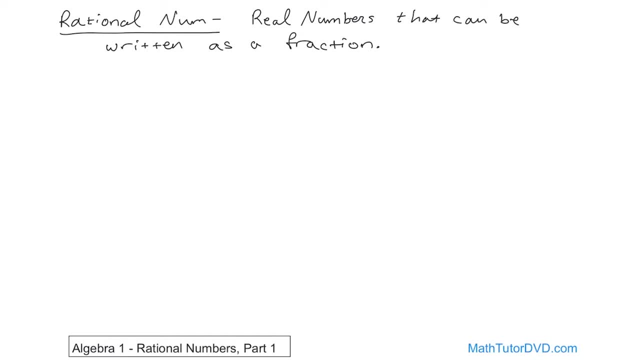 number. you can dream up Negative fractions like negative 1, half positive, 3, fourths negative decimals like negative 0.5, positive 0.8, any number you can dream of that is negative or positive. that doesn't have an imaginary i. 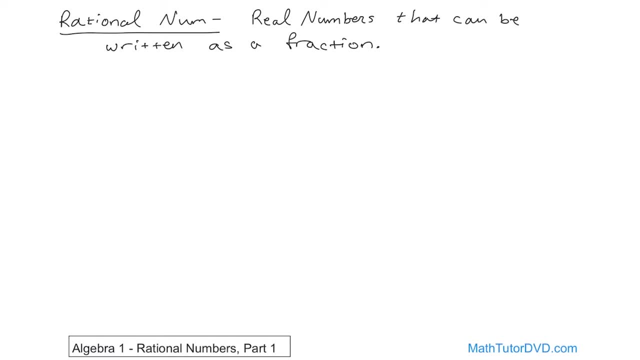 In it, which we'll talk about later. those are called real numbers. They're the tangible numbers that you can touch, Anyway. so it's a real number that can be written as a fraction. So let's give some examples of what a rational number would be. The number 0 is a rational. 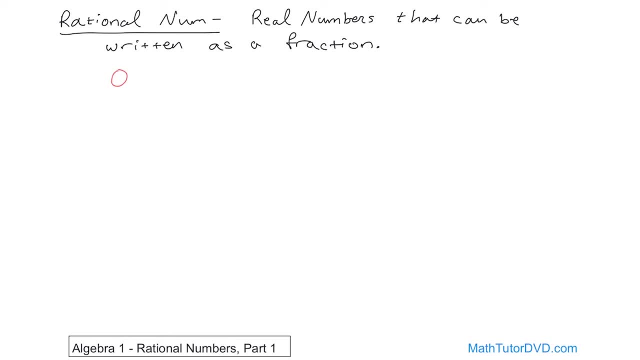 number. What you need to do is ask yourself to see if it's rational or not. Can you write this number as a fraction? How would you write the number 0 as a fraction? Well, 0 can be written as, for instance, 0 over 1, right, You could also write it as 0 over anything. 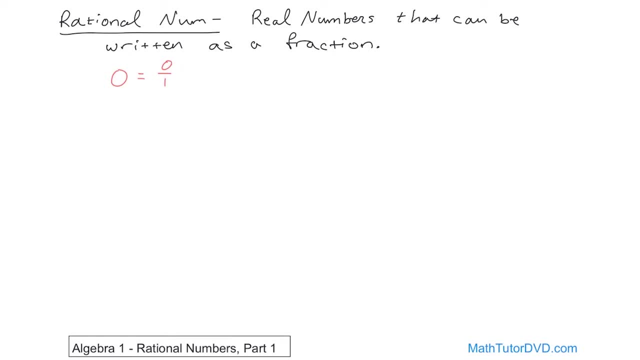 because 0 divided by anything is always going to be 0. So the number 0 is able to be written as a fraction. All you have to do is find one fraction that you can write this number as, And if you can do that, then the number is rational. So the number 0 is rational. 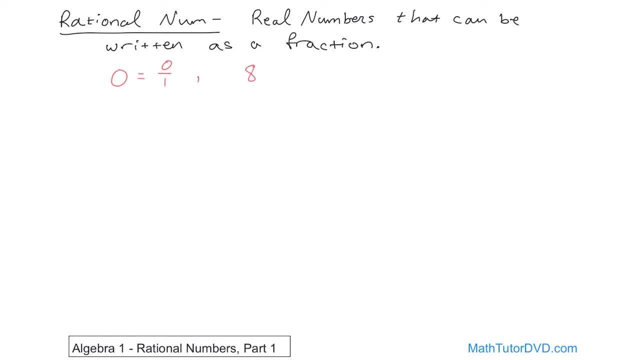 Let's take another example. What about the number 8?? Is that a rational number? Well, you just ask yourself: can I write this number as a fraction? And you think about it for a second and say, yes, I can write it as 8 over 1.. So the number 8 is a rational number. 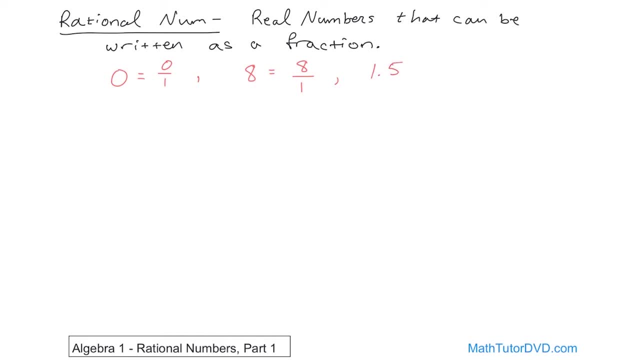 What about the number 1.5?? Is that a rational number? Well, you can write the number 1.5 as 3 halves. right, That's a fraction: 3 halves If you take 3 and divide it by 2 in your calculator. 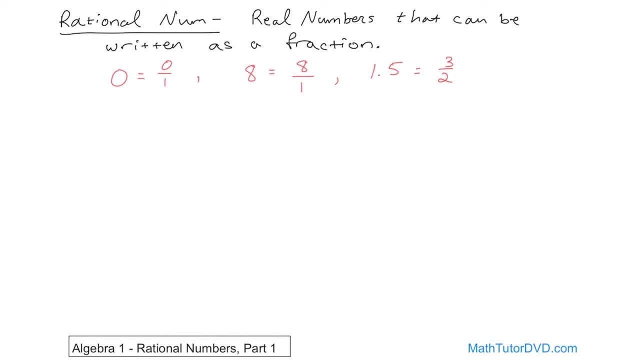 or if you do it longhand, you'll find out that you get exactly 1.5.. So the number 1.5 is rational. So you see, lots and lots of different kinds of numbers are rational. Let's pick another example. What about negative 0.67?? Now you look at something like that and 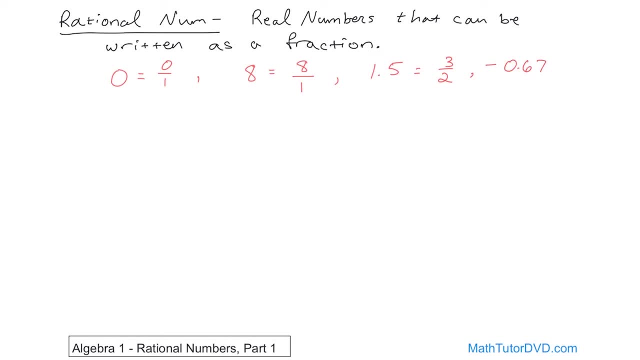 you're like: well, how would I write it? That is a fraction. Well, notice that this decimal. it stops at 0.67.. It's a negative, but it's 0.67.. There are no numbers after it. So anytime you have a number that stops. 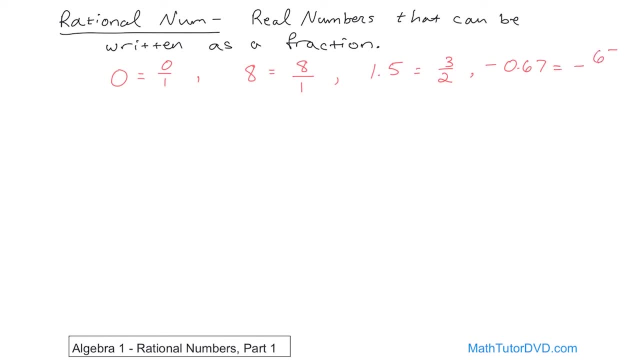 like that. the negative sign has to stay there, But you can write it, for instance, as 67 over 100. If you think about that, that's what's happening. You take the number 67, divide by 100. It's moving the decimal two spots, So you get the 0.67.. Of course, negative. 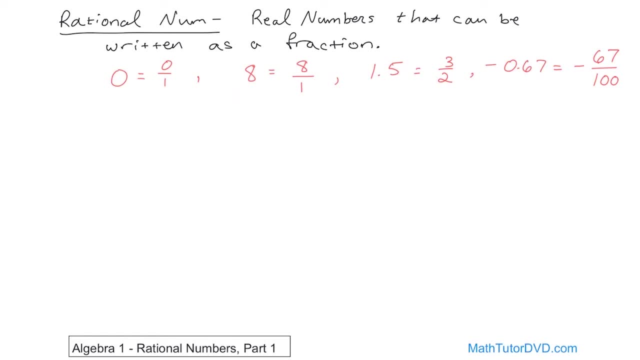 or positive doesn't matter. I'm just trying to give you a flavor for a bunch of examples. 0.. So this is how a number looks. If you do get the 0.67,, what you don't hear is: as often as you're are going to do that. No, there's just a check with your numbers. 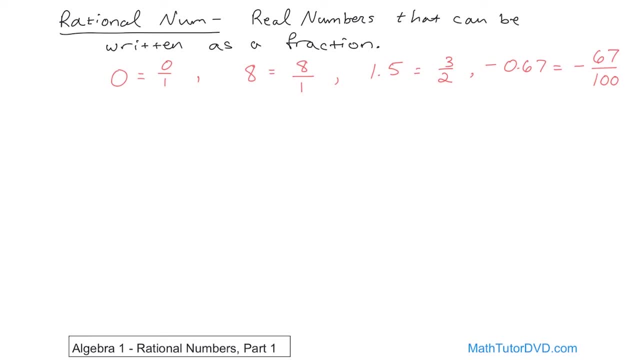 So with a decimal you write 0.67, or if you see a number that's actually moving towards thatlee, right, then that means that a function up there is missing a number. listeners answer this as you count it. that's not real. So saying RA to a negative whole number is: 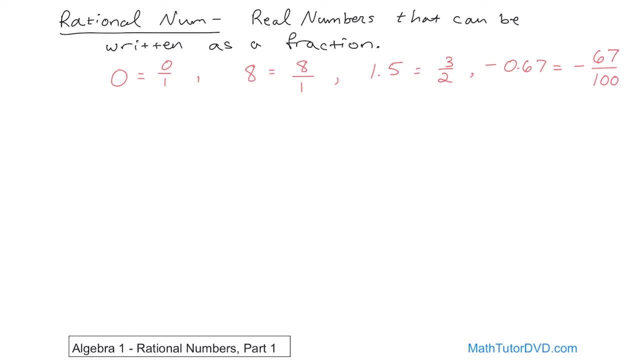 going to increase your number. Now, I didn't guess that by any chance that I had possibly rational, then what would be an example of an irrational number? right, We haven't talked about that yet. We're going to talk about irrational numbers later, but I want to give you an example. 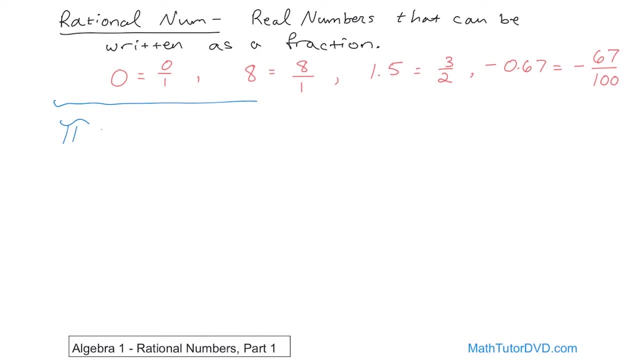 The famous number pi. you've probably heard of it right, And normally you learn that pi is equal to 3.14, and you normally stop there and say 3.14.. Well, in fact, if pi was actually exactly equal. 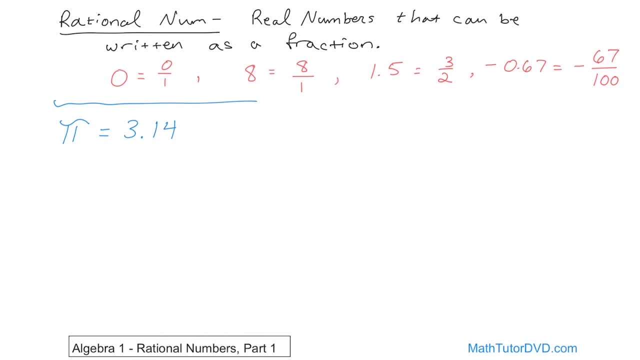 to 3.14,. you can write this as a fraction. You can write this as a fraction. In fact, you can write this as 314 divided by 100.. That would move the decimal. That would be how you'd write it as. 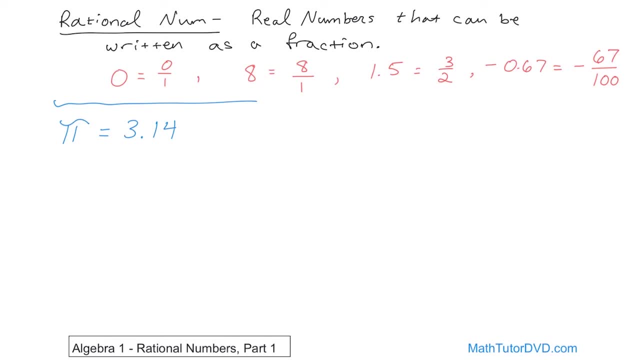 a fraction, But pi is not equal to 3.14,. no matter what you may have been taught, It's not equal to this. It's close, but it's not quite equal to this. Pi is really equal to 3.1415926, dot, dot. 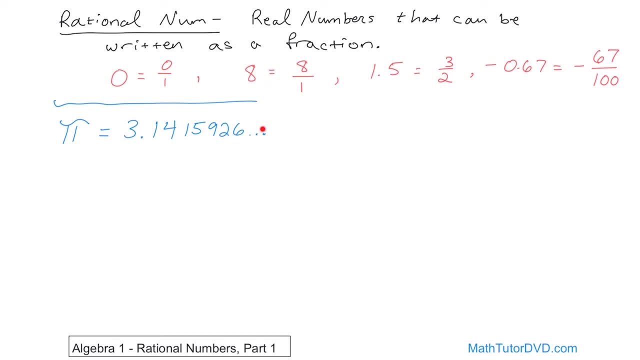 dot, dot, dot. And when I put the dots, it means that there are numbers that come after this and they go on forever and ever and ever. You see, pi is a very special number. It's irrational. It means that it has a decimal portion that doesn't really have any repeating. 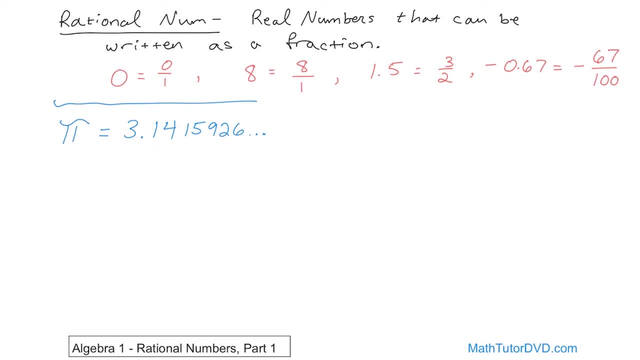 nature to it: 1, 4, 1,, 5, 9,, 2, 6.. There's no repeating nature here. These numbers, you can calculate them on for thousands and thousands of decimal places, and there really, 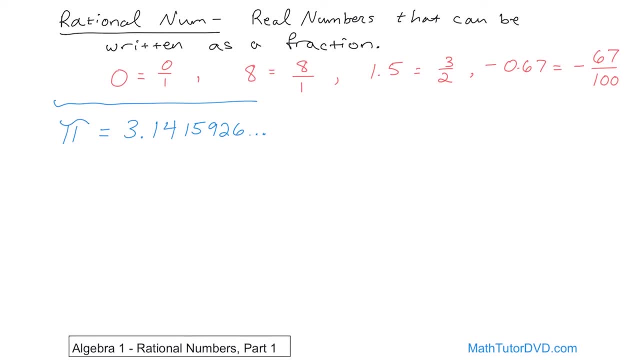 won't be any repeating patterns, So I'm kind of getting ahead of myself a little bit. but the concept of pi is this non-repeating decimal that goes on and on forever and you cannot write that as a simple fraction. You can't pull two numbers out like 10 over 2, or you might have. 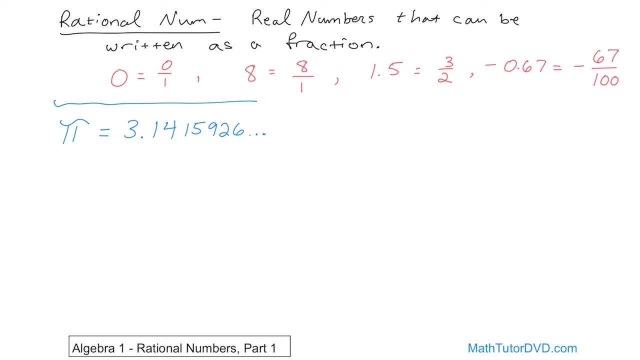 read that 22 over 7 is pi, but really that's just a close approximation. You cannot write this decimal as a fraction and that means that pi is irrational. There are other irrational numbers out there. So anyway, this lesson is on the rational numbers and we'll get to irrationals. 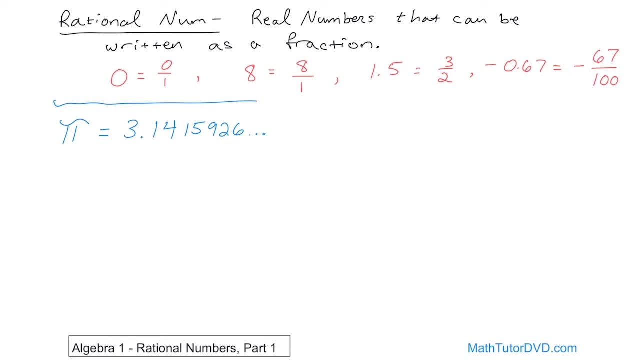 later. So what we want to do next is we want to do a little bit of practice with these things called rational numbers. So what I want you to do is fill in the following numbers or blanks with either a less than symbol, A greater than a symbol or an equal to symbol, And it's just getting you practice dealing with. 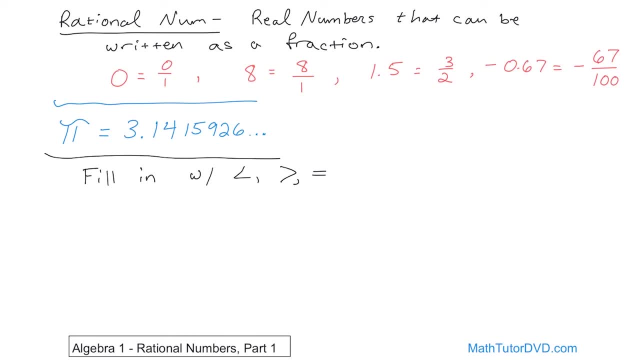 these rational numbers which we all talked about before, is known as a fraction. What if you have one-ninth and you want to figure out if that's greater than, less than or equal to four, twenty-sevenths? How would you do that? Well, you're trying to compare these two things, So you need to. there's 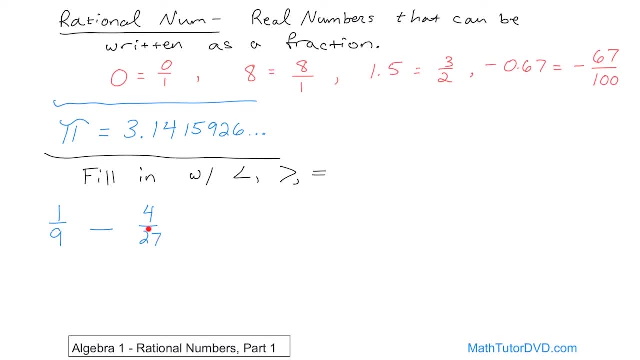 a lot of different ways to do it, but the way I teach it is: you want to get a common denominator, and so you express both fractions in the same denominator. You have 27 and you have 9, so I can multiply that by 27,, and I can multiply that by 27,, and I can multiply that by 27,. 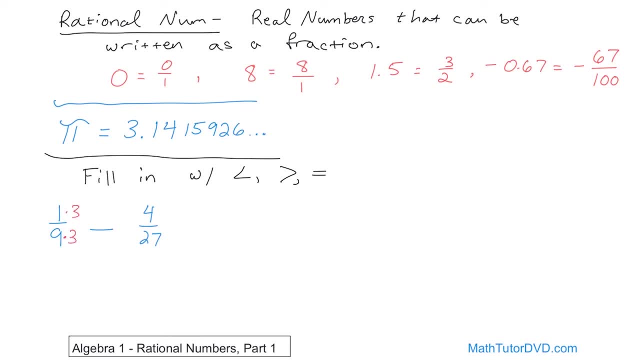 and I can multiply this fraction by 3 over 3.. And when I do that, I'm going to have a 3 over 27,. blank: 4 over 27.. Now you can look in this and say which fraction is smaller. Well, 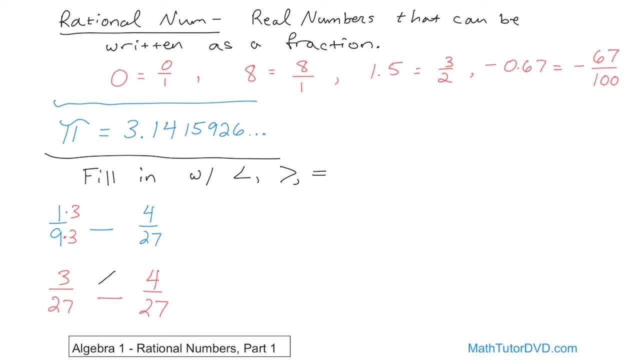 3- twenty-sevenths is smaller than 4: twenty-sevenths, so it goes like this: All right, and we're going to do all of these basically the same way. We're just getting some practice with rational numbers. What if you had negative three-fourths, blank negative nine-twelfths? 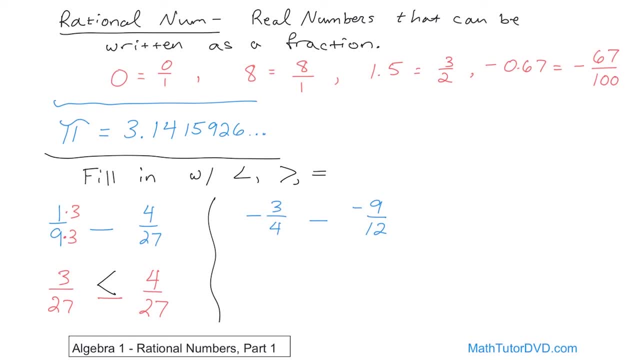 Well, the same kind of thing I want to get and work into a common denominator situation. So I have 12 and I have 4, so the way I can get a common denominator here is multiply this by 3 and this by 3, and when I do that, it'll be negative nine-twelfths blank negative nine-twelfths. So. 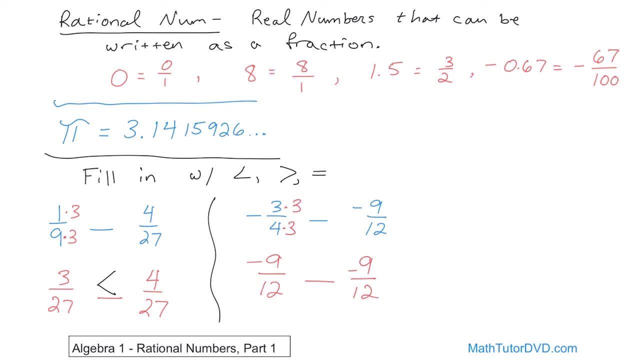 is this greater than, less than or equal to? Well, negative nine-twelfths is exactly equal to negative nine-twelfths, so it's an equal sign that you want there. That's the correct answer, And then the last one that we're going to do here is going to be three-fourths. 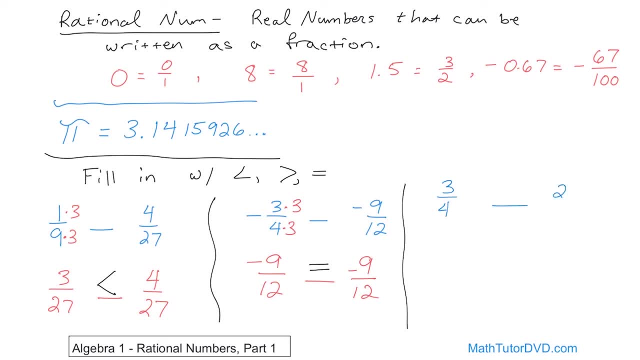 blank: 27 thirty-seconds. Same sort of thing. We want to get a common denominator: 4 times 8 is 32, so I'm going to take and multiply this fraction by 8.. So 3 times 8 will have 24 over 32.. And then 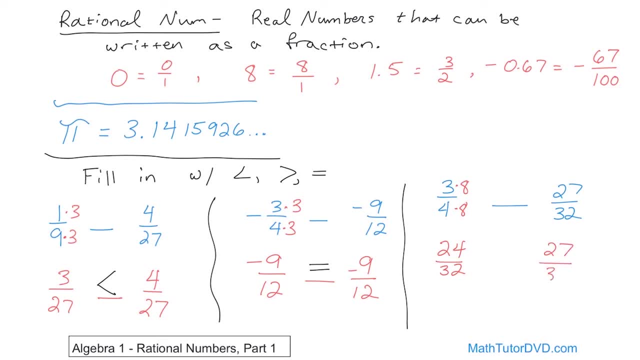 over. here it will be 27 over 32.. So now, which one's bigger? You can see that 27 thirty-seconds is larger, so the arrow's going to go this way. So in the original form, the arrow will go this way: The original fraction: whoops. this will be an equal sign. 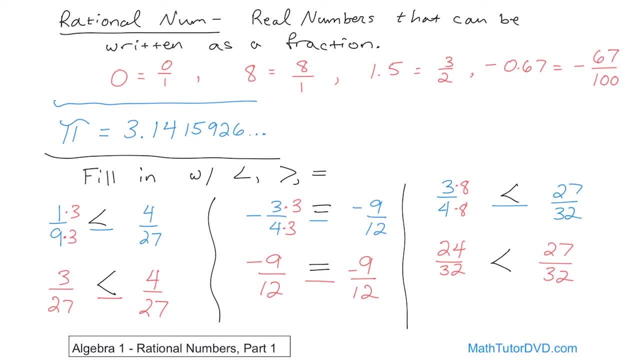 and the original fraction will go like this. So if you're trying to compare two rational numbers to figure out which one's greater than or equal to, it's best to go ahead and put them on equal footing with a common denominator. then you can figure it out. So to recap this section: 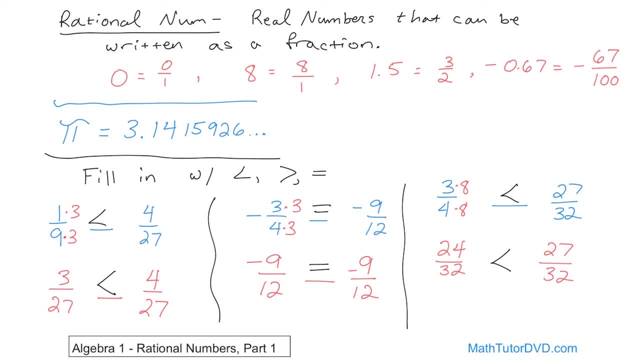 the concept of a rational number is any real number. you can dream up negative, positive, decimal, fraction or zero. that can be written as a fraction, which is almost all numbers right. Only very small numbers are written as a fraction. So if you're trying to figure out which one's 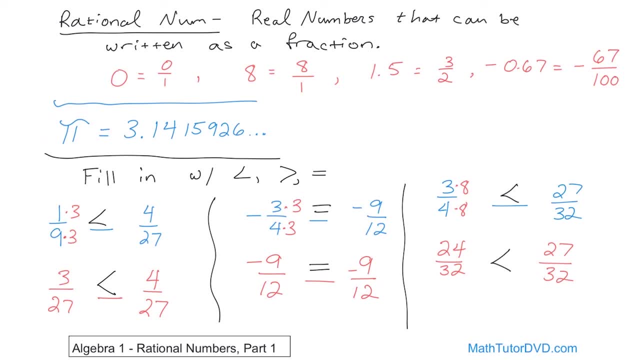 special numbers like pi are really what you call irrational. Almost everything else can be written as a fraction And to compare them we just did a few problems to show us how to do that down there. Follow me on to the next lesson. We're going to continue working. 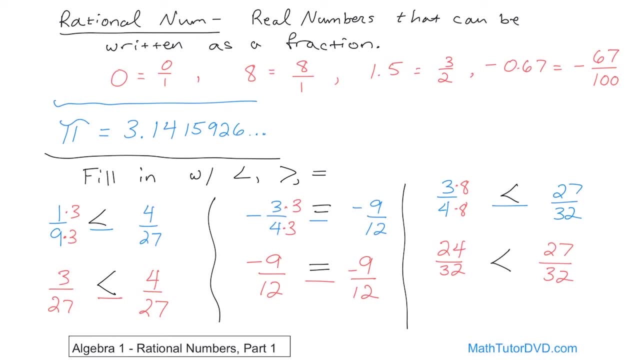 with rational numbers and learning how to deal with them in the context of algebra.